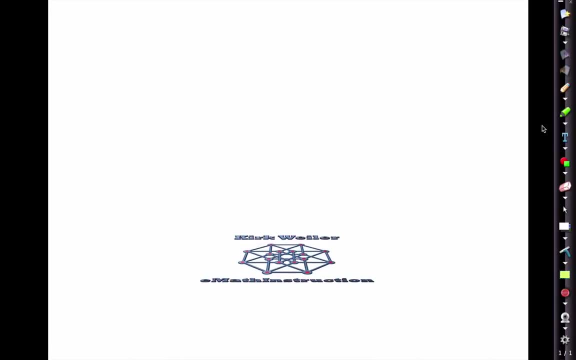 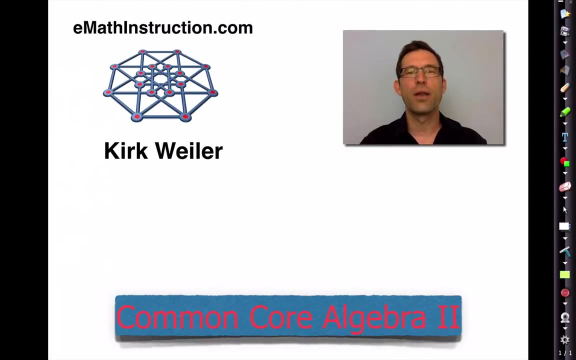 Hello, I'm Kirk Wyler and this is Common Core Algebra 2 by eMath Instruction. Today we're going to be doing Unit 4, Lesson Number 11, on solving exponential equations using logarithms. So far, the only thing we've really been able to use algebraically to solve an exponential equation. 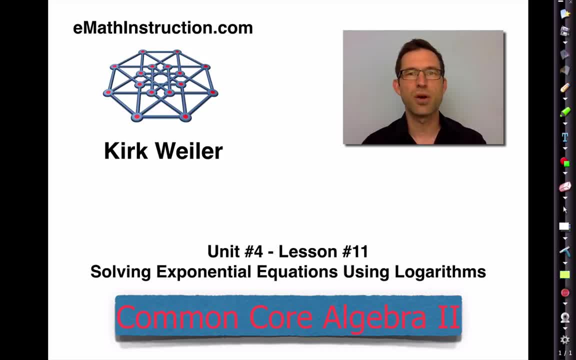 is the method of common bases. You remember that a few lessons ago where we wrote each side of the equation with the same base and then set the exponents equal. Well, that really only works if you can write both sides of the equation with the same base, And that's pretty hard in general. 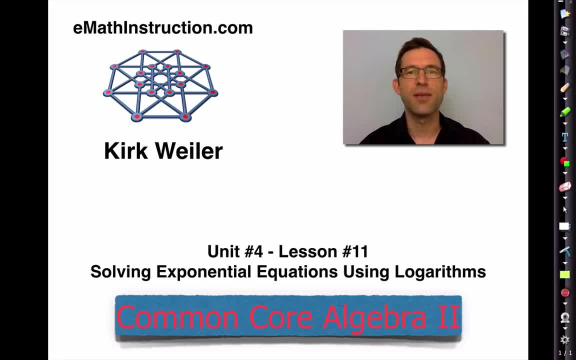 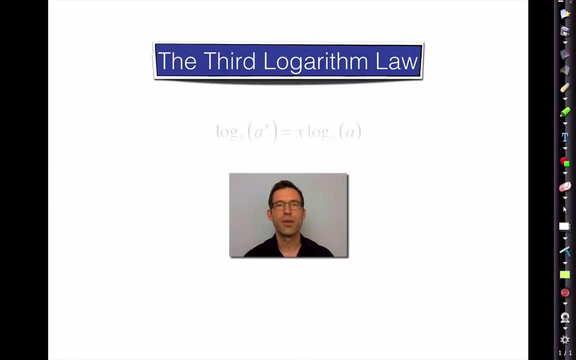 to do So today. what we're going to do is we're going to see how we can use a logarithm law to solve virtually any exponential equation. Let's take a look: The real key in everything we do today is going to be the third logarithm law. So recall that. if 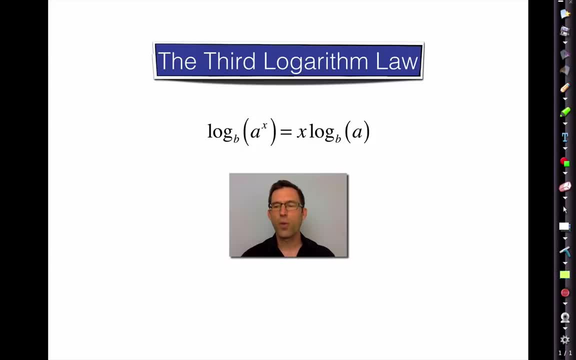 we have log base b of a to the x. we can literally bring that x out. We can take that exponent and bring it out and form a product with it. And this is pretty critical because by doing that we take the variable that we're trying to solve for, which used to be in the exponent. 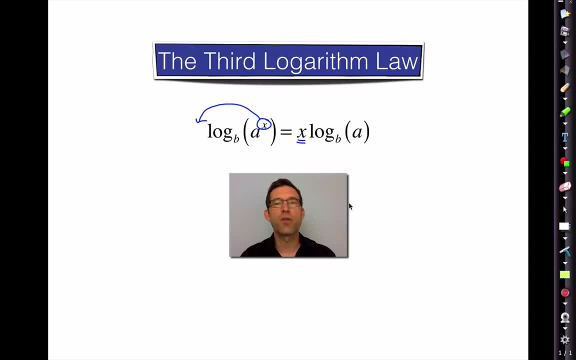 and now we just bring it on down, So it's just part of a product instead And, believe it or not, that'll make all the difference in the world in terms of solving equations. Let's just clear that out. So let's kind of see how this is done. 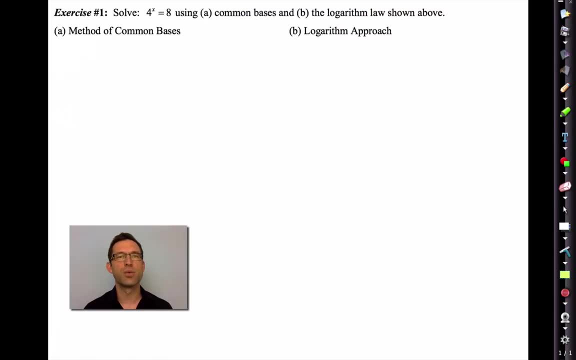 All right, Number one: we've got. solve 4 to the x equals 8 using a- the method of common bases and b- the logarithm law shown above. Well, or at least on the previous slide. So pause the video now See if you can remember how to solve this with the method of common. 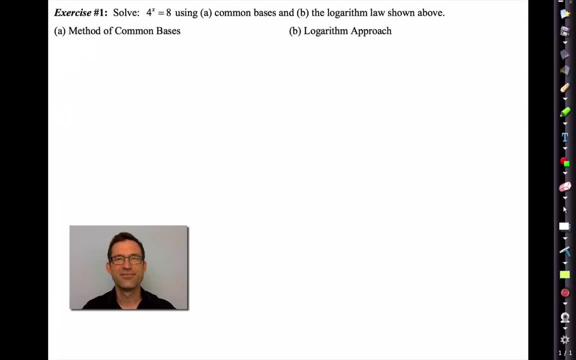 bases. All right, Let's go through it. I'm going to rewrite the problem down really quickly: 4 to the x equals 8.. Remember how the method of common bases works. I look at the 4,, I look at the 8, and I try to think of something that I can use as a common base. Well, 4 is. 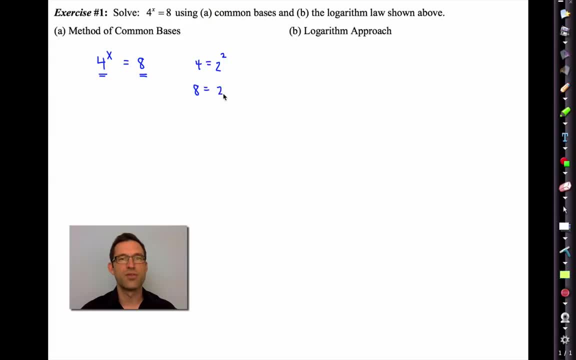 equal to 2 squared. 8 is equal to 2 cubed, So I'm going to use 2 as my common base. So on the left-hand side I'll have 2 squared. I'm going to use 2 as my common base, So on. the left-hand side, I'll have 2 squared. I'm going to use 2 as my common base. So on the right-hand side, I'll have 2 squared. I'm going to use 2 as my common base. So on the 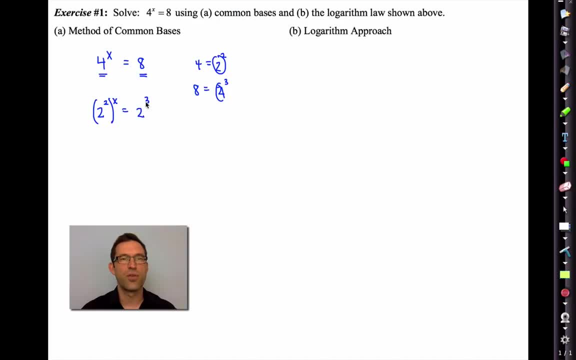 left-hand side, I'll have 2 to the 3rd, Remember. then I can use the exponent law that says that I will multiply those two exponents and get 2 to the 2x equals 2 to the 3.. And as: 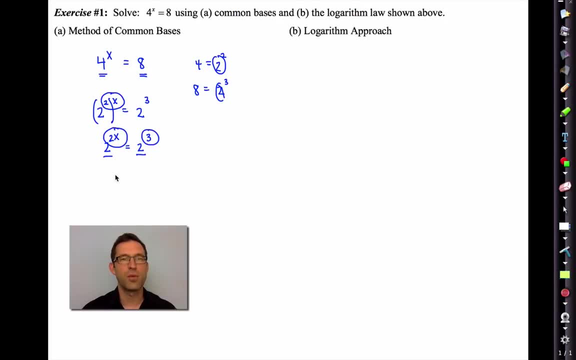 soon as we've got those common bases, we can now set the exponents equal 2 times: x is equal to 3 and x is equal to 3 halves. There we go Right, The method of common bases. But let's take a look at how we can use logarithms. 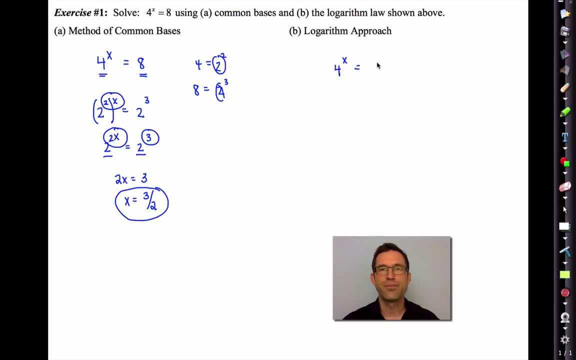 Now, of course, one of the golden rules of algebra is: you can pretty much, pretty much do anything you want to both sides of the equation, as long as you do it to both sides of the equation. So what I'm going to do is I'm going to take the log of both sides of the equation. 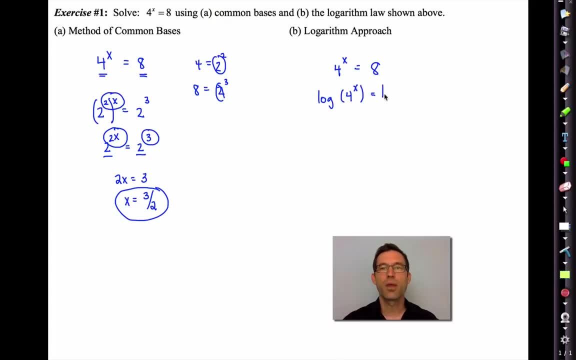 Now, what should I make my base? Well, due to the fact that the calculator has base 10, and it could have other bases, but it definitely has base 10, I'm going to use the common law. I'm going to use the common log, not the common law. 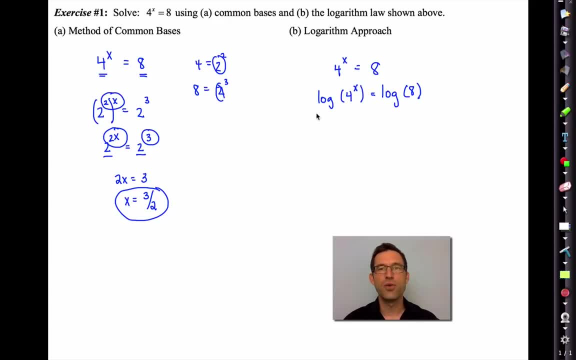 That's something totally different, And what I can now do with this logarithm is I can use that log law that pops that x out, So I'll get x and I'm going to put a little dot there. for multiplication times, the log of 4 is equal. 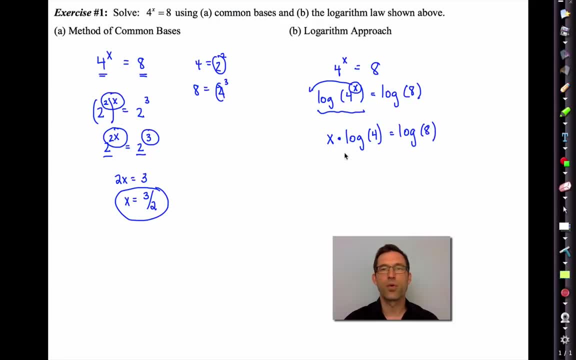 x is equal to the log of 8.. Now of course I can solve for x by dividing both sides by the log of 4.. So x is equal to the log of 8 divided by the log of 4.. Now it might be tempted to think that's the log of 2, you know. 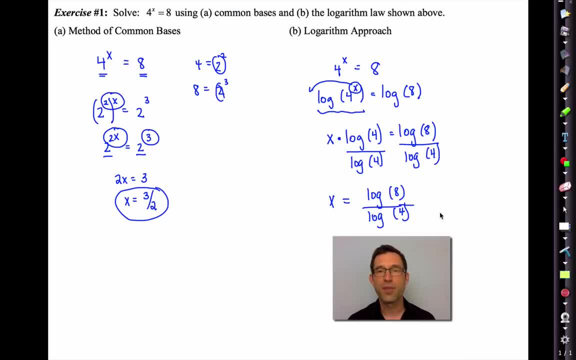 because I can do like 8 divided by 4, and I get 2,, but it's not In fact. this is where I want to use the calculator Now. I'm not going to have the TI-84 plus. 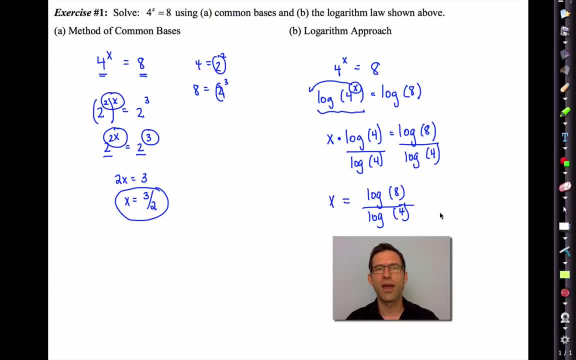 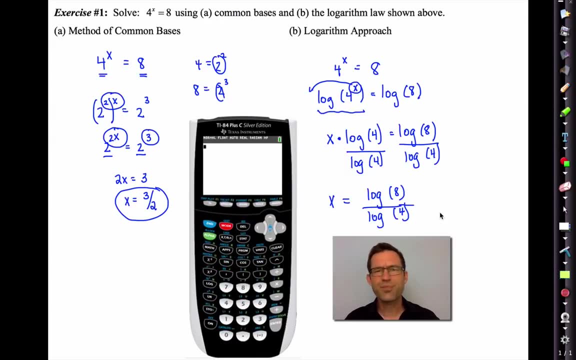 I'm going to pass open a lot today, but I do want to show you what it looks like when I enter that into my calculator. So let's just do it this one time. Hello, TI-84 plus. All right, all I'm showing you is how to evaluate the log of 8 divided by the log of 4,. 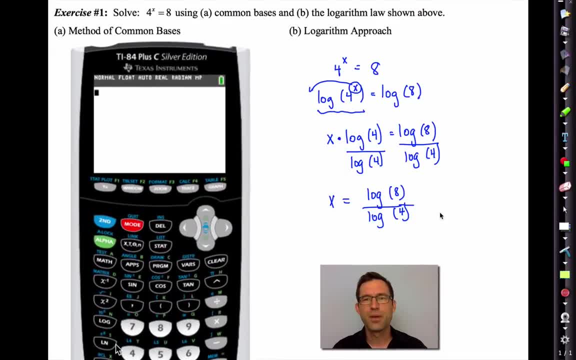 and it's easy enough, Let's do it. I'm going to hit the log put in 8, divided by the log of 4.. Got it all in there. Everything looks good. Nothing funny with parentheses or anything like that. 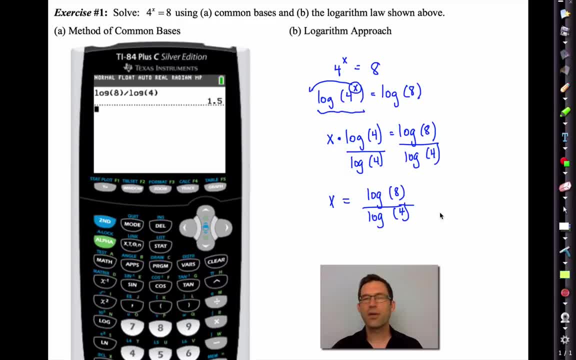 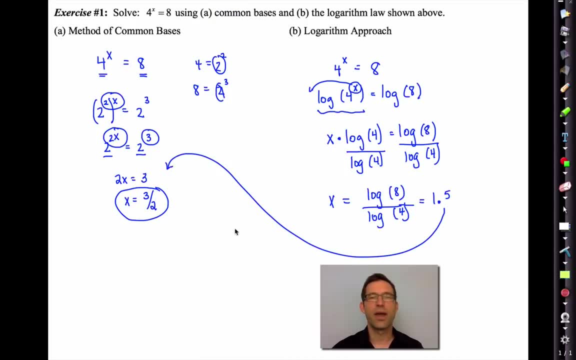 And I hit enter and look what my calculator tells me. It tells me 1.5, which is precisely what I had over here. All right, So it's really pretty impressive. you know, without using common bases or anything like that. 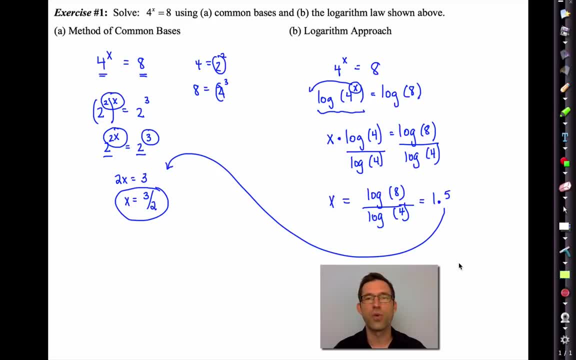 That third logarithm law allows me to solve this exponential equation very, very fast. All right, Pause the video now and write down anything you need to. Letter B is very important, So thank you. Let's think hard about what we did there. 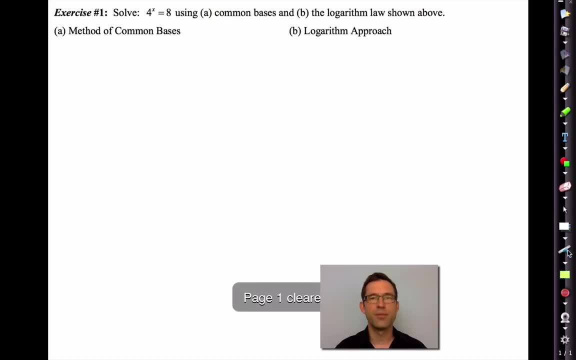 Okay, let me get rid of it. Let's keep going, All right. exercise two: Solve each of the following equations for the value of x. Round your answers to the nearest hundredth. All right, well, again, let me do the first one with you, okay. 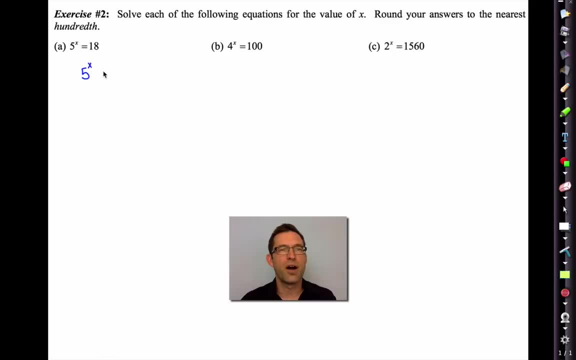 And then I'll have you work on some of the other ones on your own. So we get 5 to the x equals 18.. I'm going to do the log, The log of both sides. Now. don't skip this step. 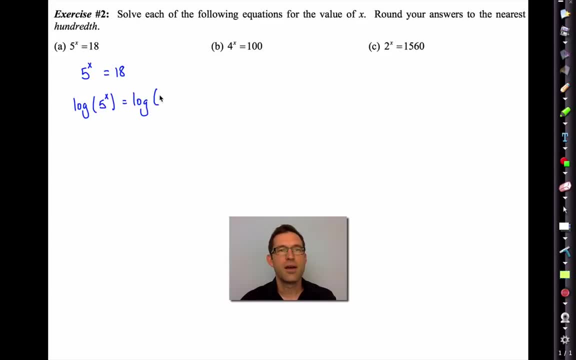 Some students want to go immediately to the next step and I guess that's okay, but I think it's really helpful to have this step first, The next step, where that x comes out right: x times the log of 5 equals the log of 18,. 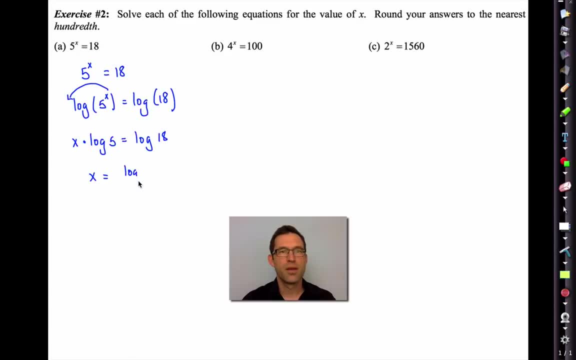 right. So x is equal to log 18 divided by the log of 5.. And if I put that in the right place, I'm going to get the log of 18 divided by the log of 5.. And if I put that in the right place, I'm going to get the log of 18 divided by the log of 5.. 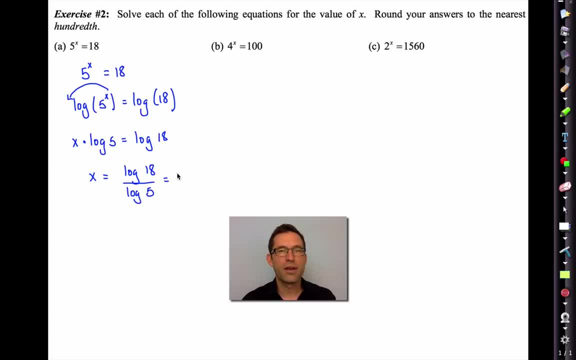 If I put that into my calculator, just like I did before, what I'll find out is that's approximately 1.80.. It's kind of cool, isn't it? That means 5, never forget to. the 1.80 is 18.. 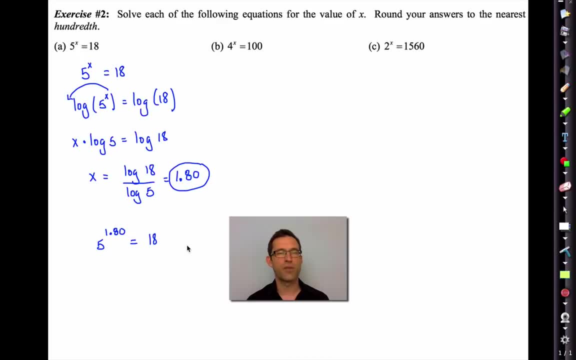 Kind of makes sense: 5 to the first is 5.. 5 to the second is 25.. So whatever 5 had to be raised to get 18 had to lie between 1 and 2. And it did. It was 1 point, you know roughly 8.. 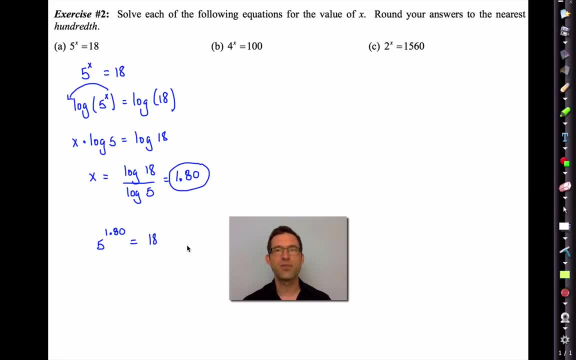 Alright, why don't you try letters B and C? pause the video now and take a couple minutes. Alright, let's take a look at them quickly. Take the log of both sides: log of 4 to the x equals log of 100.. 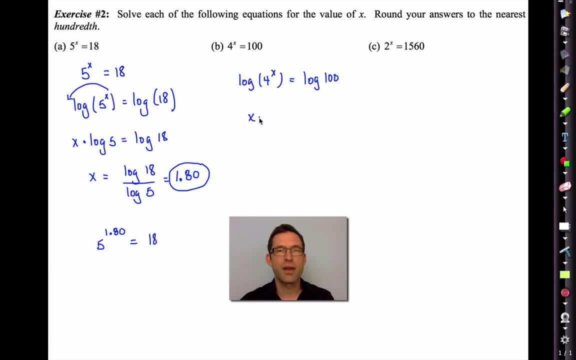 By the way, the log of 100 is 2,, but we don't even have to think about that. I can pop that x out now. the x times log of 4 equals the log of 100, and x is the log. 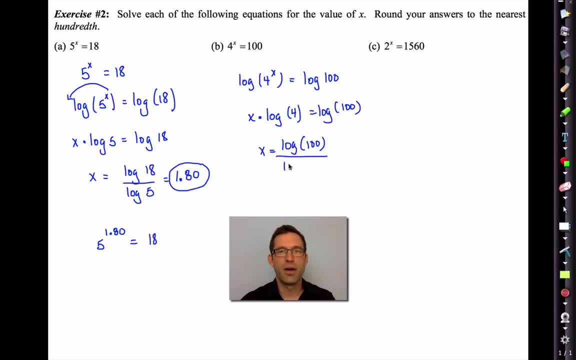 of 100 divided by the log of 4, which if we work that out on our calculator can't do it- in my head is about 3.32.. Alright, you can kind of see how this is all going. The log of 2 to the x equals the log. 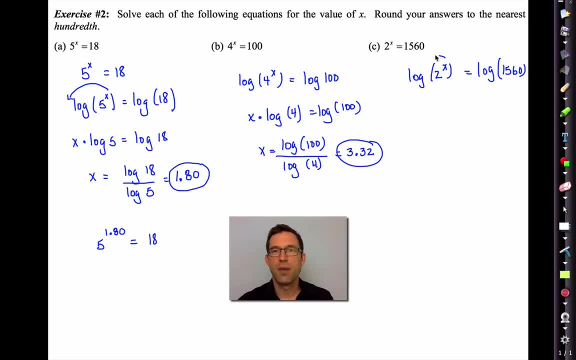 The log of 1560, pop the x out x times. log of 2 equals the log of 1560, and x equals the log of 1560 divided by the log of 2, which ends up being what About 10.61.. 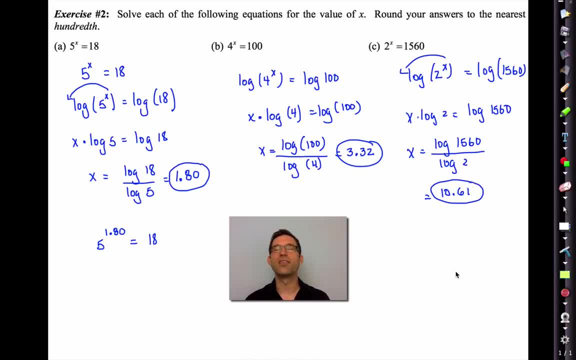 Alright. Now, of course, if that, If that was the entire deal, if the whole deal was, that's it, well then, the lesson would be over and we would call it a day. But we can do a little bit more with this, so let's keep going. 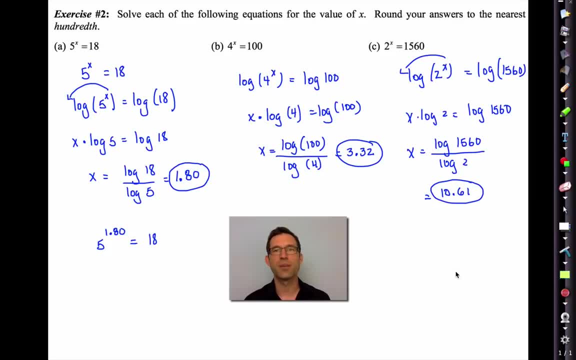 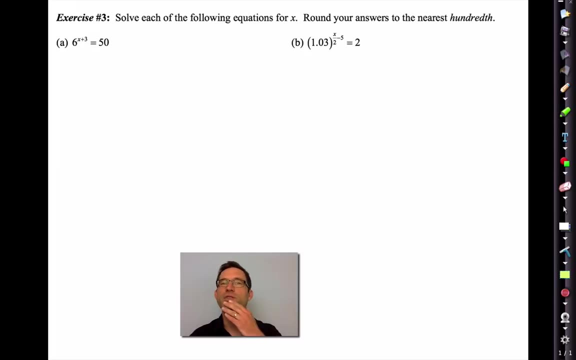 Pause the video now. write down anything you need to, and then we'll take this up a notch. Alright, here we go. Okay, Solve each of the following equations for x: Round your answers to the nearest hundredth. Alright, Now I'd like you to take a look at both of these two equations for a moment. 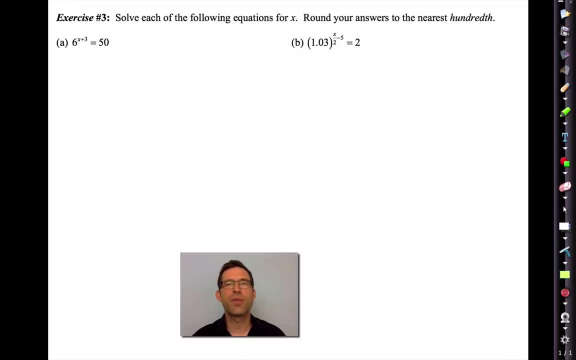 Okay, The big difference between these equations and the ones we were dealing with before is that they're more complicated. The exponents are more complicated, So I want to be more careful. I don't want to introduce any rounding errors or anything like that, and yet I'm still going. 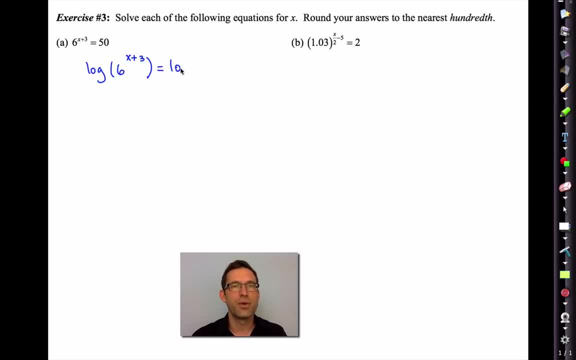 to do exactly what I did before. I'm simply going to take the log of both sides. Let's work through the first one together. Then that x plus 3 is going to come out front. Now this is critical. Keep that x plus 3 in parentheses, okay. 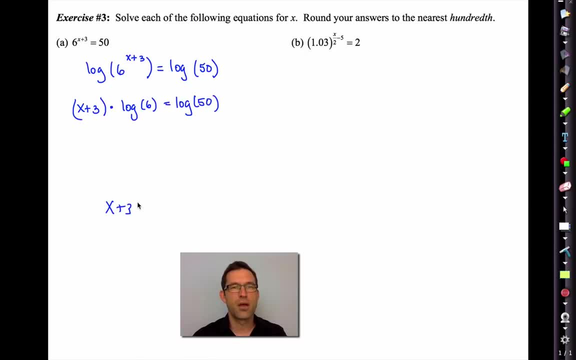 If all I do is write this right as my left side, then it's only the 3 that's multiplying by log 6. And that's not the case. It's the entire x plus 3.. So we have to be very careful there. 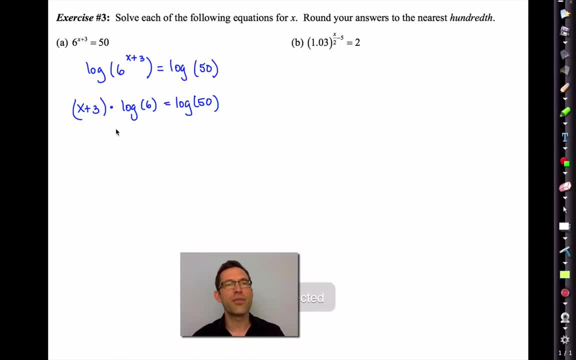 Alright, Now how do we get the 3?? Or how do we get the x all by itself? Well, think about this: I've taken x, I've added 3, and then I've multiplied by log 6 and gotten log 50.. 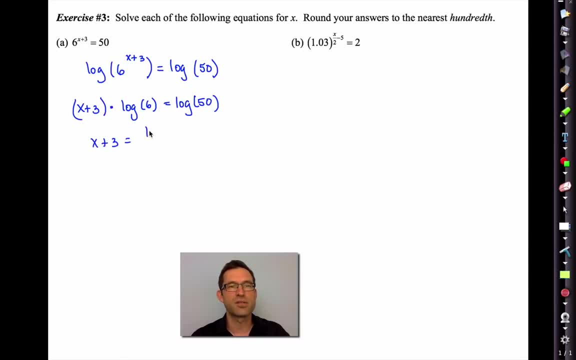 So the first thing I'm going to do is get rid of the multiplication by log 6 by dividing by log 6.. Now you could evaluate that on your own. You could evaluate that on your calculator, But I wouldn't. I would just leave it. 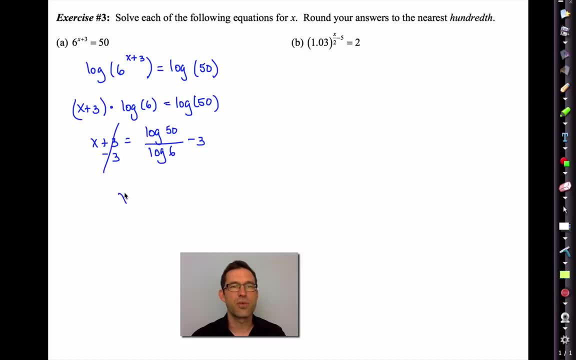 Because then I will get rid of that plus 3, right Like that. Then I'll enter all of this on my calculator at once: Log of 50 divided by log of 6 minus 3.. Now, if you haven't already tried this, try this really quick, and then I'll give you. 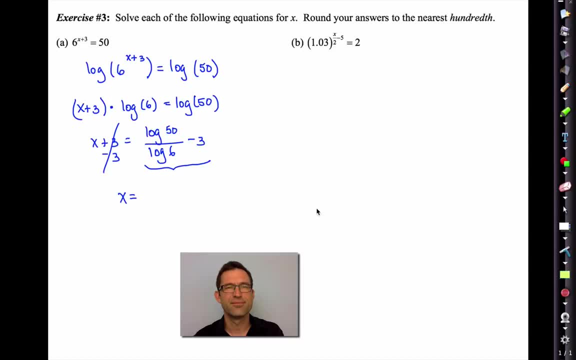 the answer so you can check yourself. Alright. Well, if you work through all of that, what do we end up getting? It's negative. We should get negative 0.8.. where are we? Yeah, negative 0.82, about. 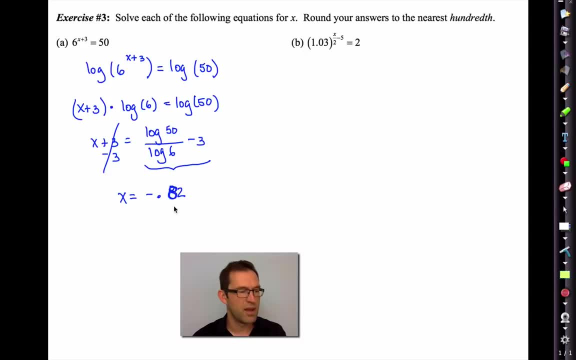 Again, can't do these in your head. impossible. Negative 0.82.. Let's try this one: Very, very similar, A little more challenging: Alright Log of 1.03 to the x divided by 2 minus 5.. 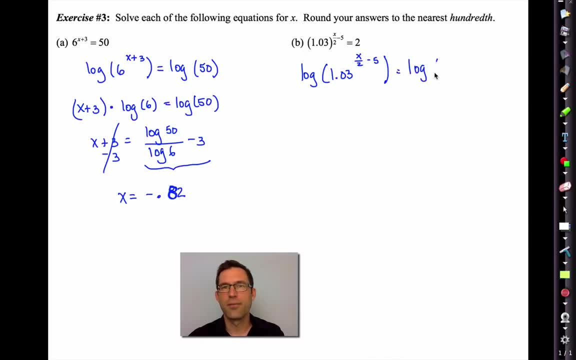 Alright, x divided by 2 minus 5 equals the log of 2.. Again, just like before we can bring this out, Let's keep it in parentheses: x divided by 2 minus 5 times the log of 1.03 equals the log of 2.. 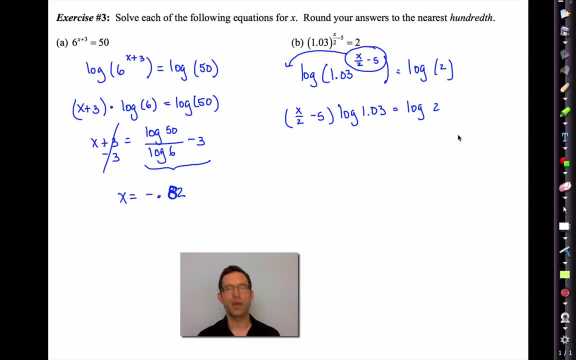 Now again, I really want you to understand when we look at this equation and we think I'm solving for x. let's talk about how to do it. We took x and we divided by 2, then we subtracted 5.. 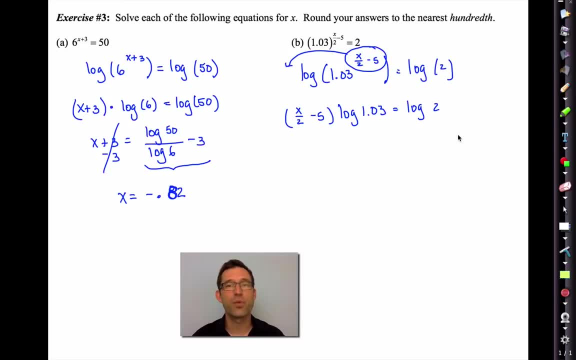 Then we multiplied by log of 1.03, right? So we can easily undo this by first dividing both sides by log of 1.03.. You don't want to distribute that log of 1.03.. Just want to divide by it on both sides to get rid of it. 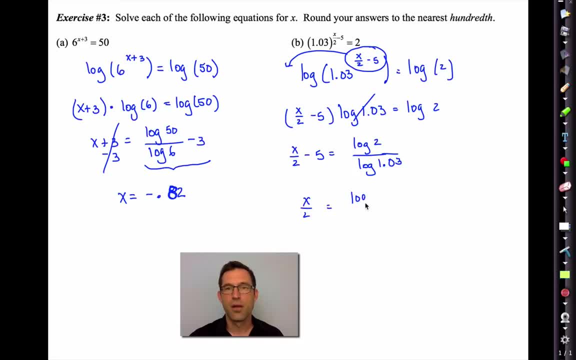 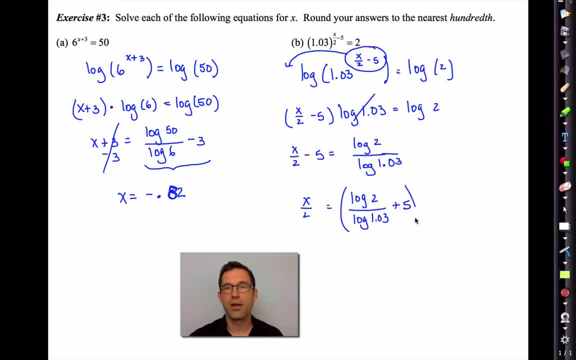 and then we're going to multiply the entire quantity by 2.. Now, that's your final answer, Not in decimal form, but it's your final answer. The issue now is just evaluating it, and you might want to evaluate it slow. 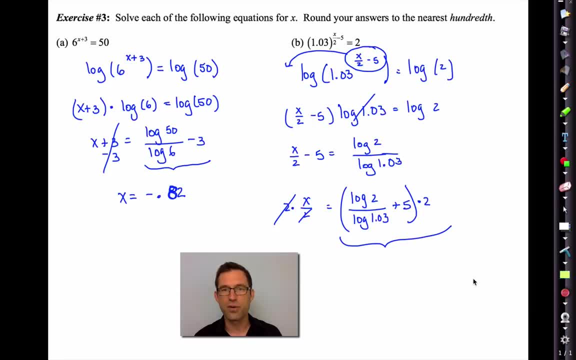 You might want to do log 2 divided by log of 1.03, enter plus 5, enter times 2, enter Right, so you can do it in phases. That's okay, but it's critical that you get the calculator work right. 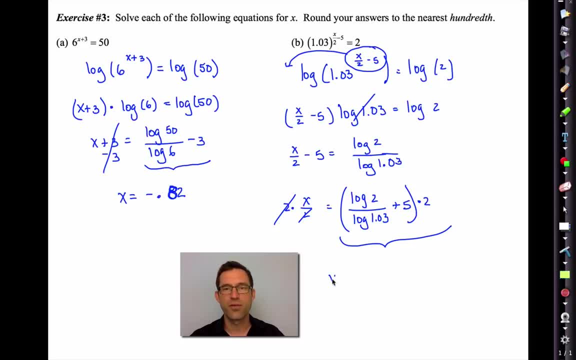 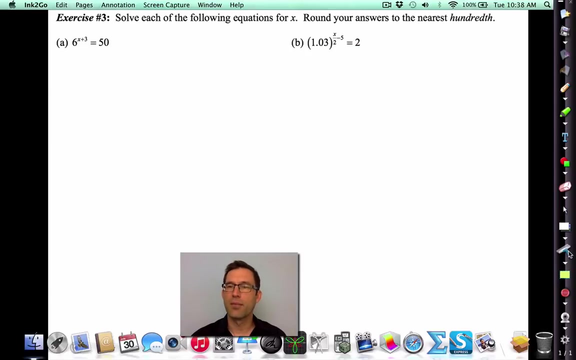 And if you do, you end up getting an answer for x. It's about 56.90, much larger than our last one. All right, So pause the video now and write down anything you need to. All right, clearing it out and moving on. 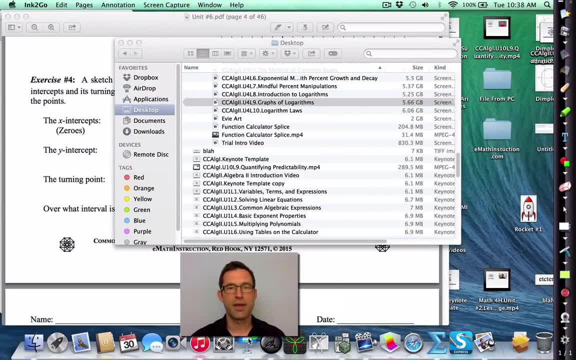 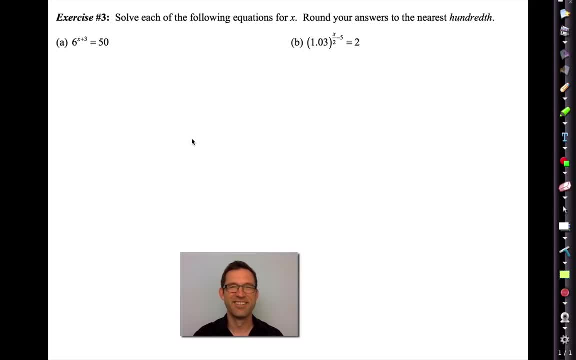 Uh-oh, We got to get back into that, that keynote. There we go. My apologies for that. You saw the inner workings of my Macintosh. All right, let's take a look at more of a modeling problem. I never understand why that happens. 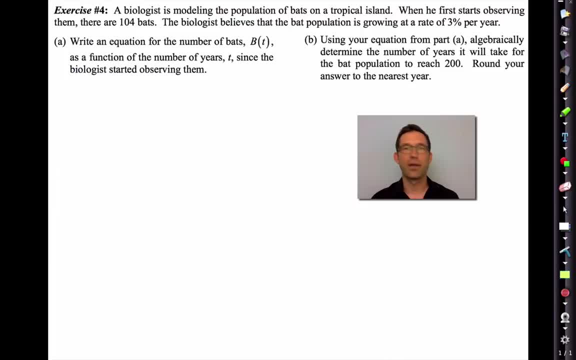 A biologist is modeling the population of bats on a tropical island. Okay, cool enough. When he first starts observing them, there are 104 bats. Okay, The biologist believes that the bat population is growing at a rate of 3% per year. 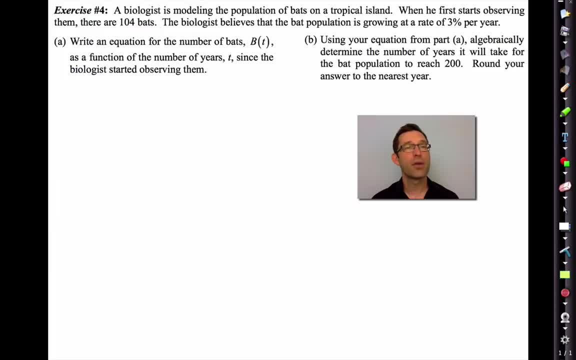 Ah, I feel some exponential modeling coming on. Letter A says: write an equation for the number of bats B of T as a function of the number of years T since the biologist started observing them. So this is something you should feel very. 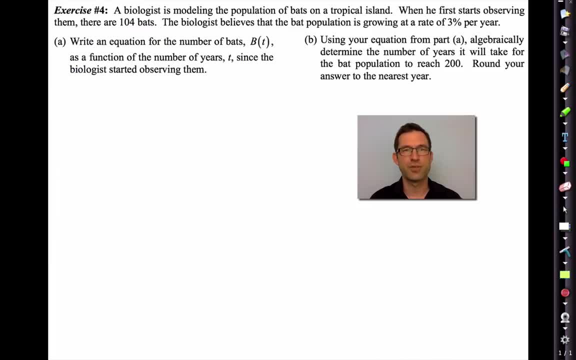 very comfortable with. Why don't you go ahead and try to write that function? All right, Hopefully, because it wasn't that long ago. Hopefully this was a piece of cake. We know we start with 104.. That's our y-intercept. 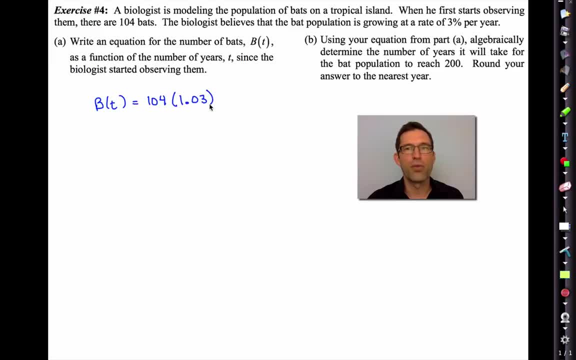 We know that every year we get to multiply it by 1.03 because it's growing at 3% per year, And then we raise it to the T. All right, simple enough. Letter B says, using your equation from A, algebraically: 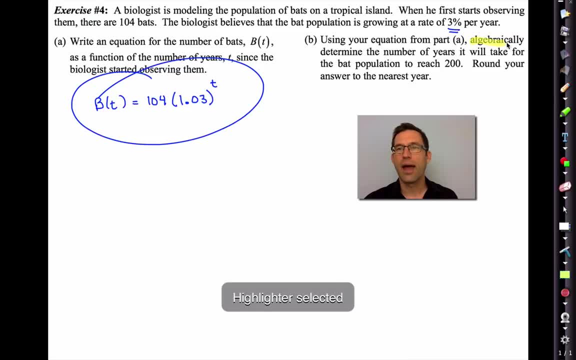 that's a very, very important word. We all know that right Algebraically determine the number of years it will take for the bat population to reach 200.. Round your answer to the nearest year. Well before we would have had to have done this graphically. 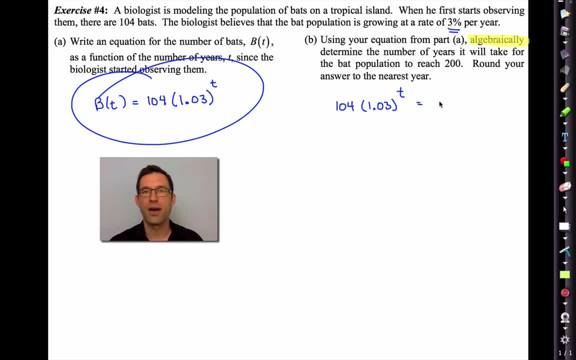 And it's kind of a pain to do it graphically, I mean, it's not terrible, but kind of a pain. Right, We'd have to put this in this, in graph: get a good window, use the intersect command, et cetera. 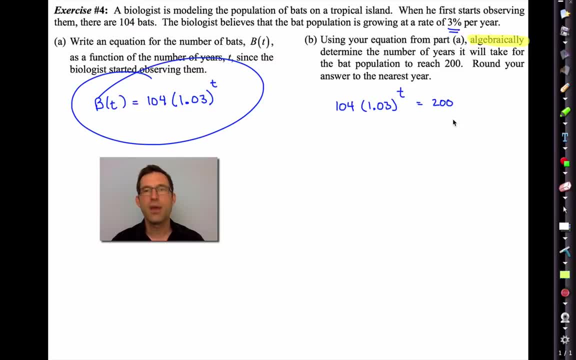 But now let's take a look at this. We want to solve for T Now. given that what we've been doing- we keep taking the logarithm as our first step, it would be an understandable thing to just say: I'm going to take the log of both sides. 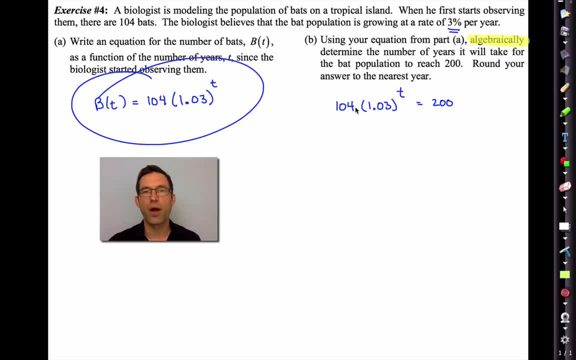 Let's pop that T out, But the problem is we've got this product here first. So the best thing to do, honestly, is to begin to solve this problem by dividing both sides by 104.. Okay, So that we have 1.03 to the T equals 200 divided by 104. 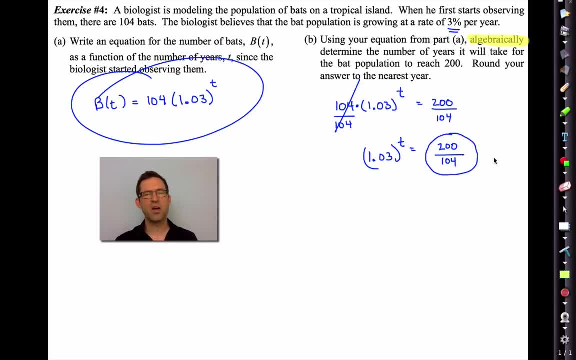 Now, if this is a nice number in terms of a decimal, you know, go ahead. even if it's not a nice number, you could use the decimal version. I'm going to leave it at that. I'm going to leave it as the fraction, all right? 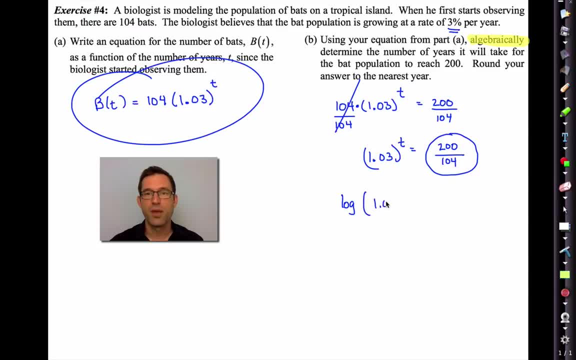 And I'm now going to take the log of both sides. So I'm going to take the log of 1.03 to the T equals the log of 200 divided by 104.. Now, of course that's going to pop the T out. 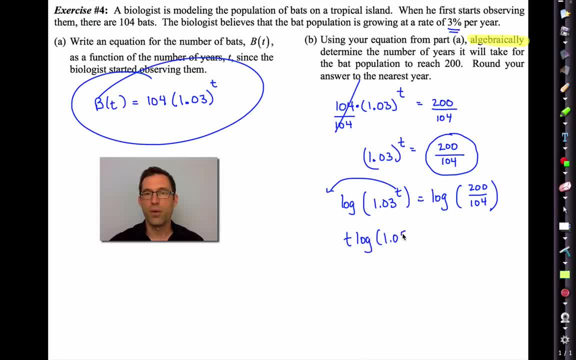 So I'll have T times the log of 1.05 equals the log of 200 divided by 104.. So now I can divide both sides by a log of 1.05.. Again, be careful, We've got two divisions going on here, one that's inside of a log. 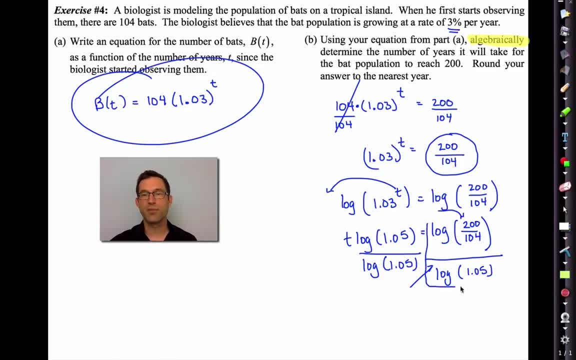 one that's sort of outside of the log. But ultimately you just have to put this all into your calculator. Why don't you go ahead and try to do that? Pause the video if you need to Throw that into your calculator and make sure you can get the right answer. 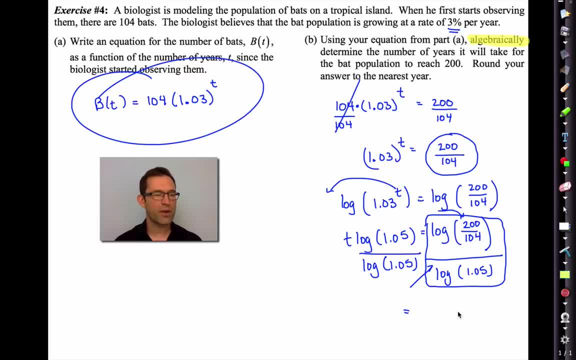 All right, well, when I crank that all into my calculator, I get an answer that's about 22 years. Twenty-two years it'll take to reach a population of 200.. All right well, they're not growing very fast. 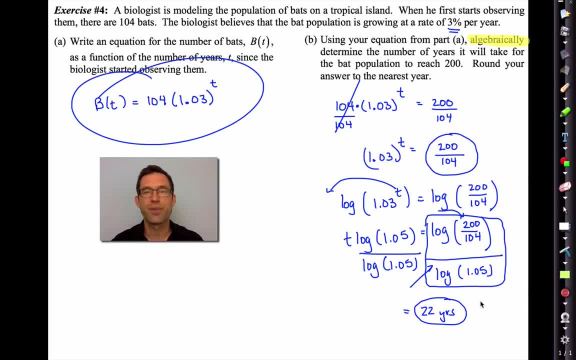 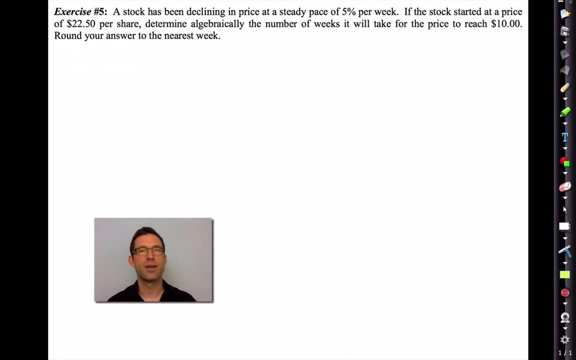 only 3% per year, but I can buy 22 years. Pause the video now and write down anything you need to. Okay, let's go ahead and do that. All right, Let's clear out that text, All right. Exercise number five: a stock has been declining in price. 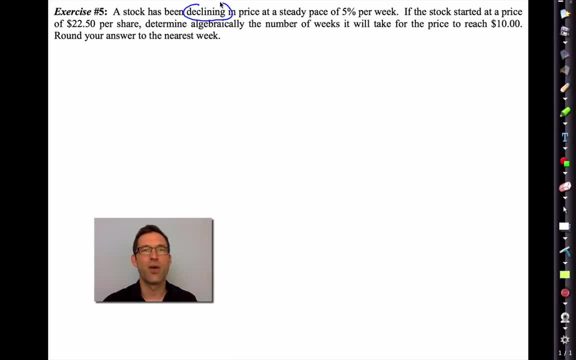 Ooh, that's important. The fact that its price is going down, declining At a steady pace of 5% per week- Okay, If the stock started at a price of 22.50 per share, determine the number of weeks it will take. 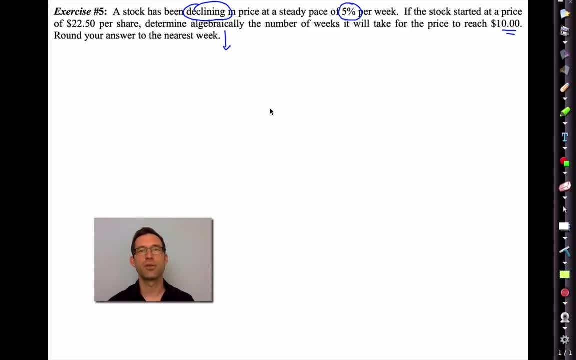 for the price to reach $10.. Round your answer to the nearest week, All right. Well, there's a couple pieces here, right, We have to model the problem and then we have to actually solve some kind of an equation. So see if you can model this problem in terms of you know. 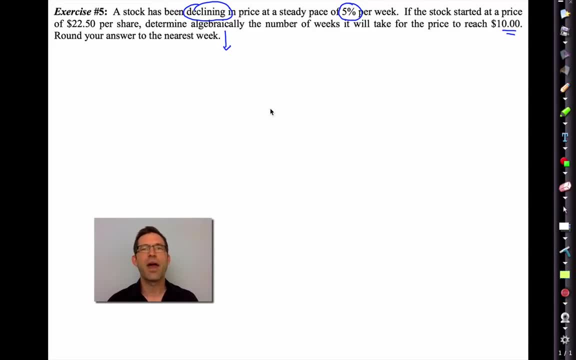 a function that models the price of the stock, and then a little bit of algebra. okay, Take a minute, or even more than a minute. All right, Let's do it. Well, if we wanted just a function that predicted the price, 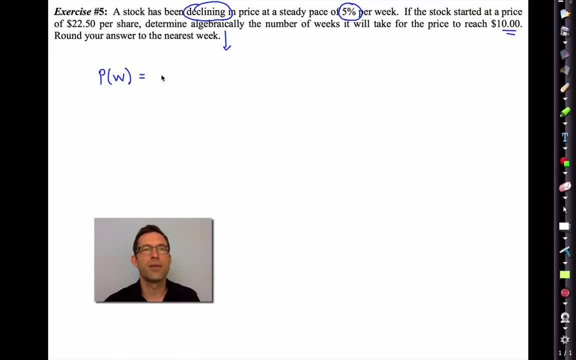 of this stock as a function of the number of weeks. right, We know it starts off at 22.50.. We know it goes down 5% per week. But remember how we accomplish that is not by multiplying by .05 or 1.05 or negative .05, but by multiplying by .95, right. 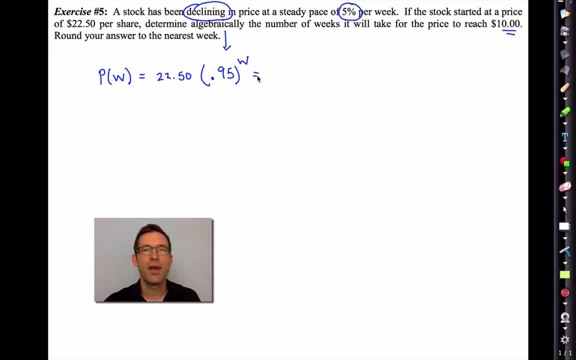 We have 95% of the price every week. Now I'm going to set that equal to $10.. And again, just like in the last problem, we could solve this graphically, but the problem specifies for us to do it algebraically. 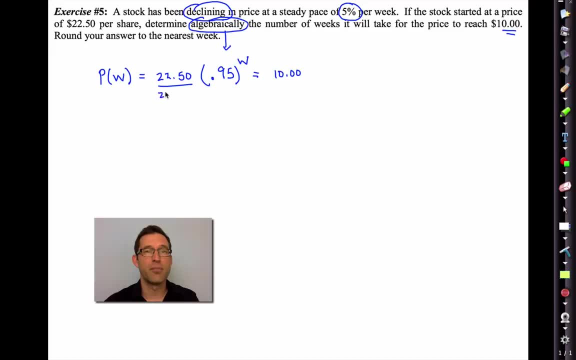 And it's a very, very similar solution. I'm going to divide both sides by 22.50.. And, just like before, if we want to deal with the decimal version of this, we can. We just wouldn't want to round it. 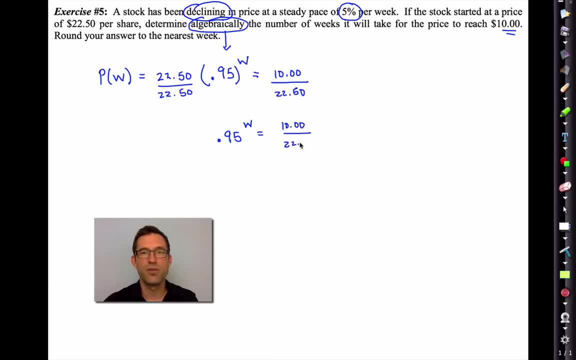 I'm going to leave it as 10 divided by 22.50.. And then I'm going to take the log of both sides And I can leave that fraction absolutely unevaluated. inside of the parentheses, No need to figure out what 10 divided by 22.50 is. 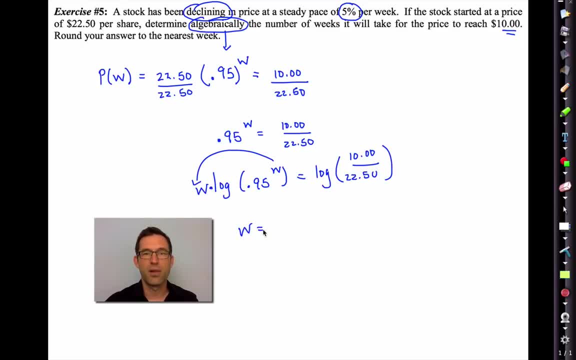 The W would pop out And then I would divide by the log of .95.. So, whew, at the end of the day we end up having this And again I would suggest to pause the video right now. Make sure you're good in terms of getting that into your calculator. 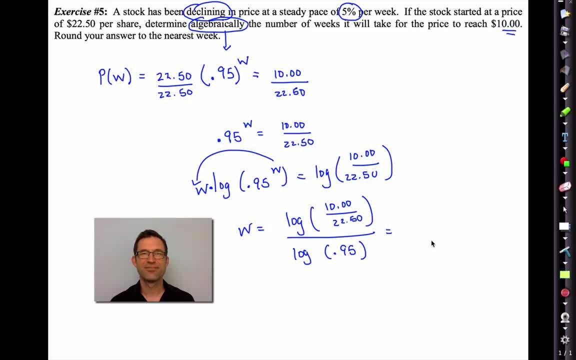 And then I'll give you the final answer. All right, Well, let's do it. Our final answer is just about 16 weeks. It'll take for that price to get down there. So pause the video now. Write down anything you need to. 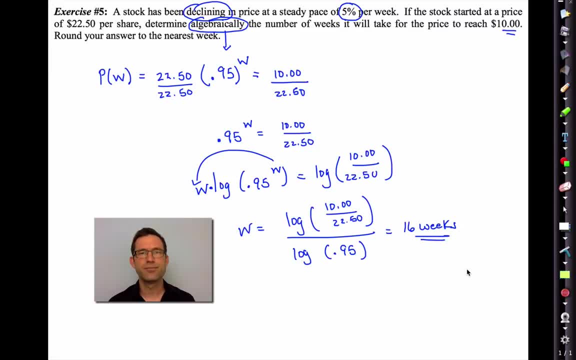 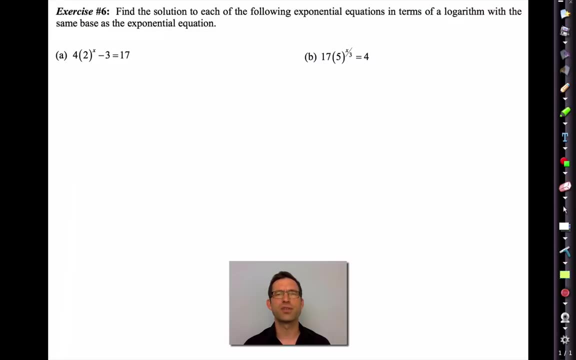 And then we'll do one last problem. that's a little bit different. All right, Let's get rid of it. One of the things that the common core would like you to be able to do is solve exponential equations and leave them in terms of logarithms, so not get a final answer like x equals 17,. 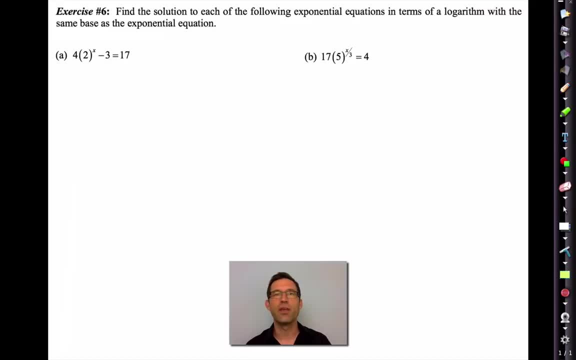 but get an answer like x equals 17.. X equals the log base 3 of 5, you know something like that. So exercise number 6 says: find the solution to each of the following exponential equations: find in terms of a logarithm: 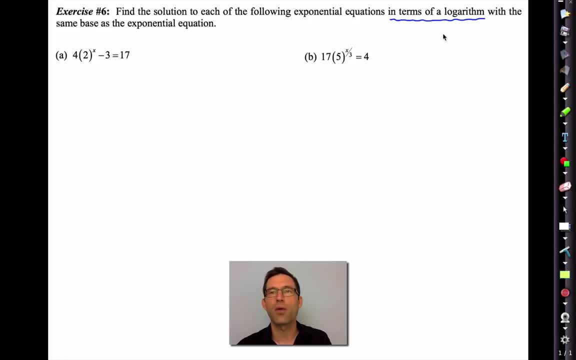 So when you see something like this, what it means is that there will be a logarithm. in your final answer It says in terms of a logarithm with the same base as the exponential equation. All right, Well, let's see how it plays out. 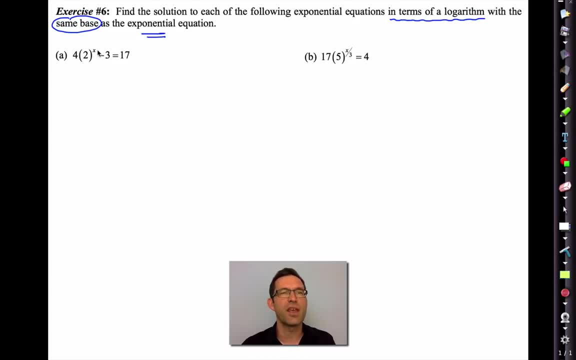 Let's solve this equation Now. take a look at what we have. We've got 2 raised to the x, then we're multiplying it by 4, then we're subtracting 3, and we're getting 17.. So the last thing I did was subtract 3, so the first thing I'm going to do is add 3.. 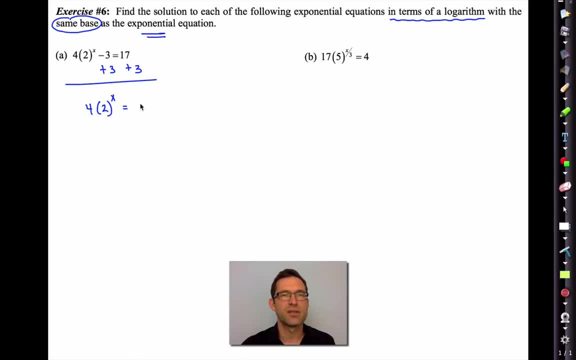 So I'm going to get: 4 times 2 to the x is equal to 20.. Right, Then I've got to get rid of that multiplication by 4, so that's easy enough. I'll just divide by 4, and I'll get: 2 to the x equals 5.. 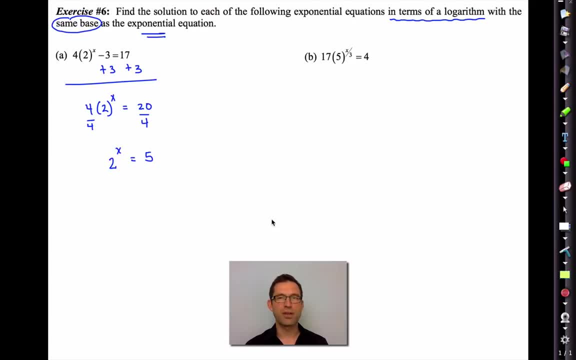 Now, what do they mean by solve this equation in terms of a logarithm? So the same base. Well, what they want me to do is do the log base 2, right, the same base of 2 to the x. 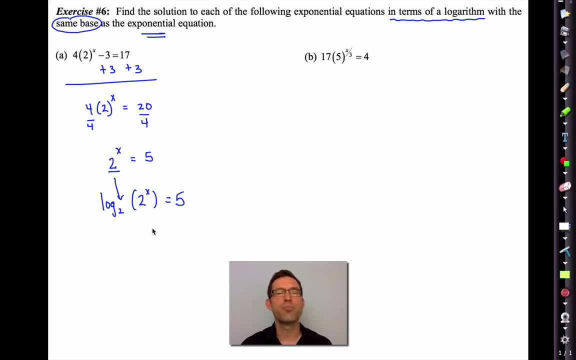 Well, now I could bring the x out. I could But think about this for a minute. The whole point of logarithms is that they're inverses of exponentials. They literally cancel These cancel Whoops. Oh, That was horrible. 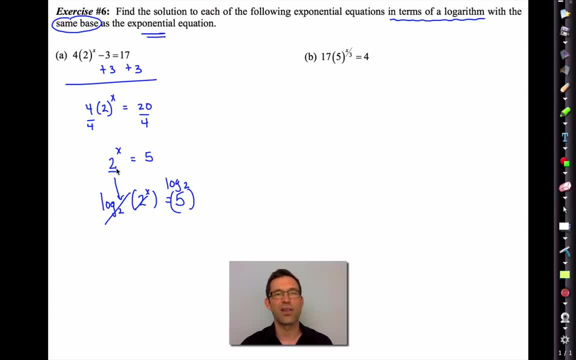 I have the log base 2 of 5 on that side. I can't take the log on the left and not the log on the right Anyway, so eventually I just get: x equals the log base 2 of 5. And that is what it is. 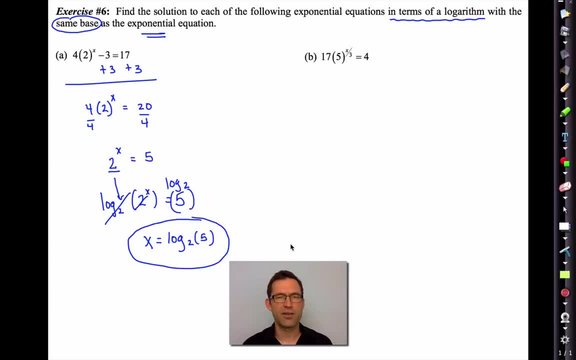 You know it's some decimal answer, but we're going to just leave it like that, okay. Very similar letter b. Okay, look at this. We've got 5 raised to the x, divided by 3 times 17, equals 4.. 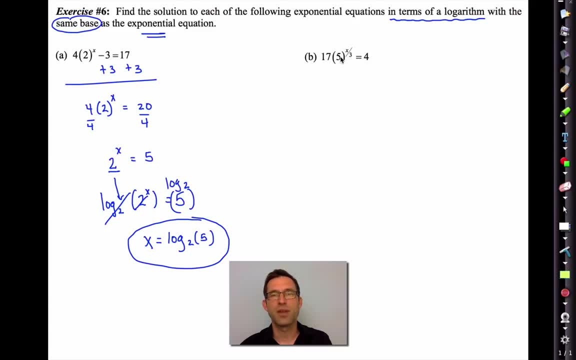 So the first thing that was done to x is we divided by 3, then we exponentiated it, then we multiplied by 17.. So the first thing I'm going to do is get rid of the 17.. So I have 5 to the x divided by 3 equals 4 17ths. 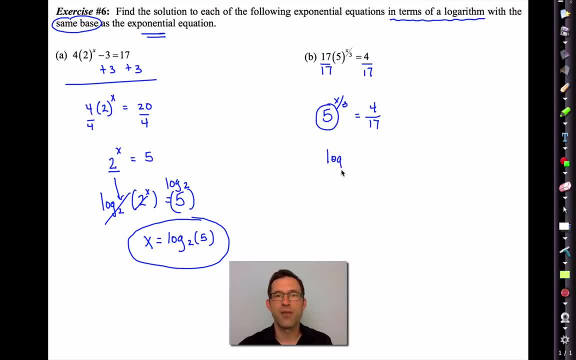 Now again, we want to rewrite the final answer in terms of a log, with the same base as what we have. So I'm going to do the log base 5 of 5 to the x divided by 3 equals the log base 5 of. 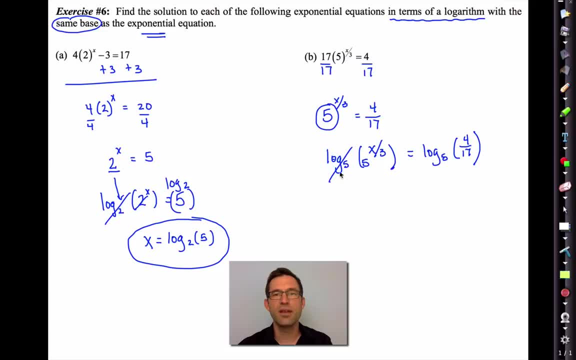 4- 17ths. Now again, the idea is that these just cancel and we're left with x divided by 3 is the log base 5 of 4- 17ths. And then, of course, I can multiply both sides by 3 and get 3- log base 5 of 4- 17ths. 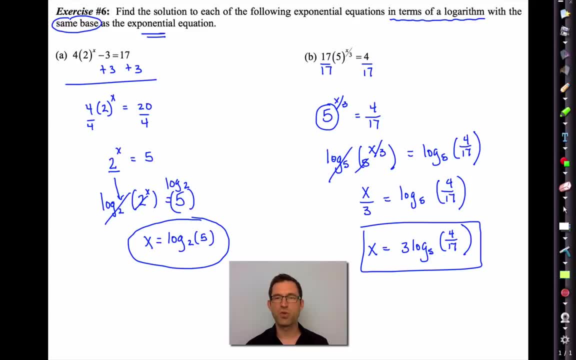 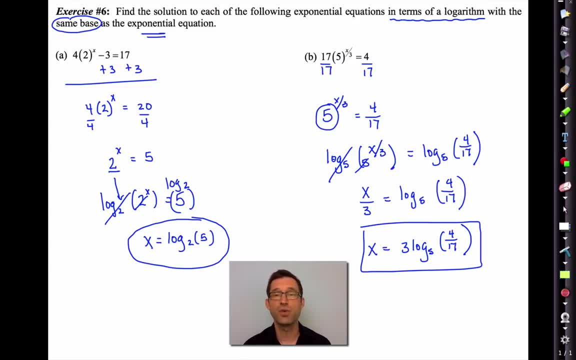 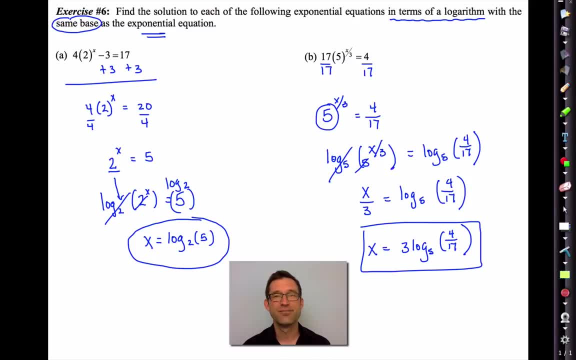 Okay, Okay, Okay. So it's not bad to have your answers like this. Okay, we'll pause the video. I'm going to clear out the text and we'll wrap up the lesson. Okay, let's do it. Text is cleared. 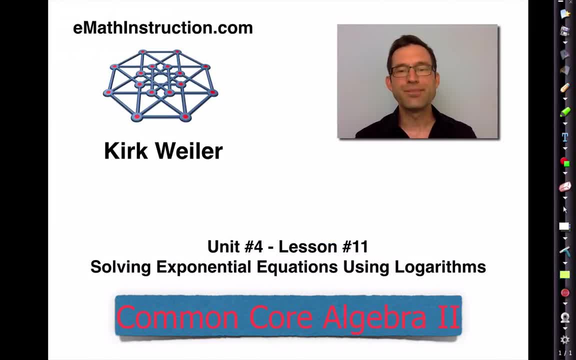 Let's finish up. So, in my personal opinion, the third log law is the most important of them all for one specific reason: It allows you to solve exponential equations algebraically. Right Now, we can solve almost any equation graphically, so we always have.